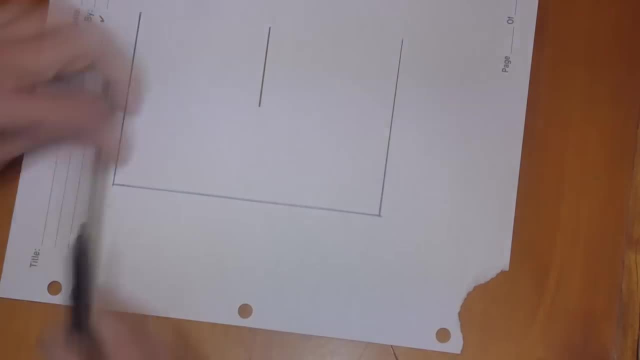 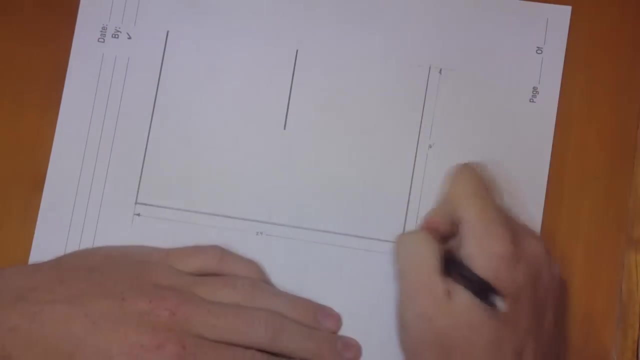 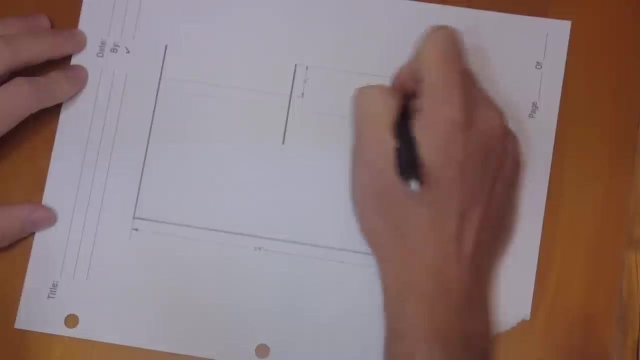 structures by causing uplift, pressure, seepage and changing the strength characteristics of soil, among other things. We have fancy computer models that do a good job simulating groundwater flow. now, but even today, one of the most important tools used by geotechnical engineers is the flow. 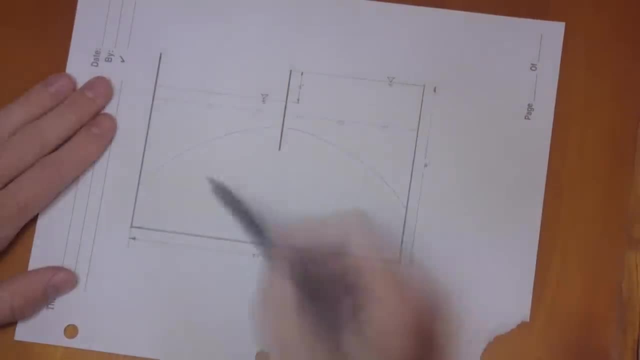 net. Without getting into the nitty-gritty details, a flow net consists of two sets of perpendicular lines which create a curve. The flow net consists of two sets of perpendicular lines with a linear grid. One set are equipotentials, or lines which connect points with the same. 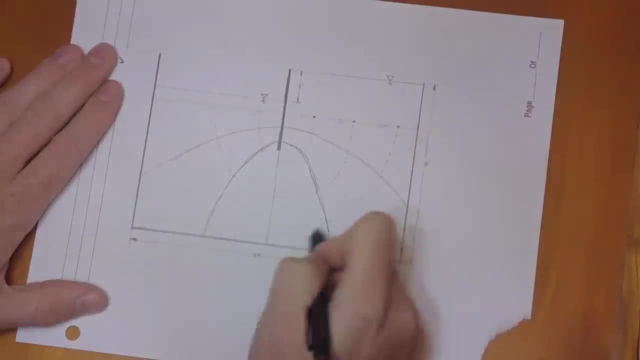 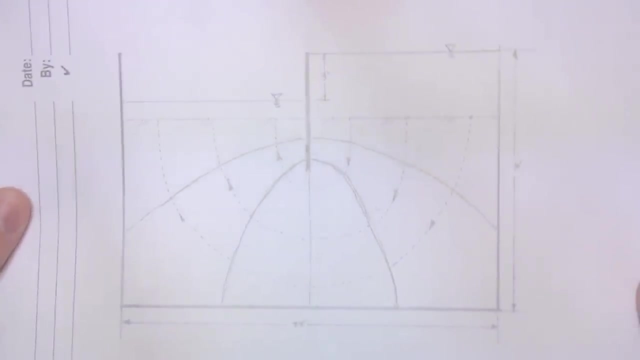 pressure. Once the equipotential lines are drawn, the flow lines are just drawn perpendicular to them, forming squares. These kind of simplified drawings make pretty pictures, but do they really reflect how groundwater flows in real life? It's always important to ground truth your calculations. 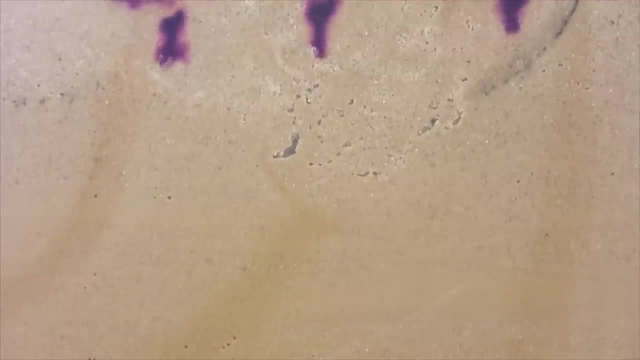 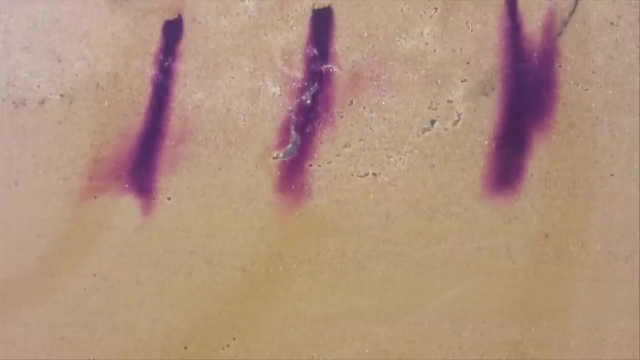 sometimes even with real ground. This model is designed to do just that: It simulates the flow of groundwater, but it's not always the case. The flow net is designed to simulate the flow of groundwater around an obstruction, to illustrate the morphology and velocity of the flow. It's 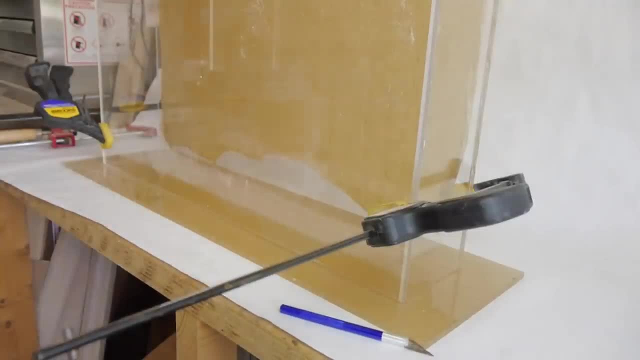 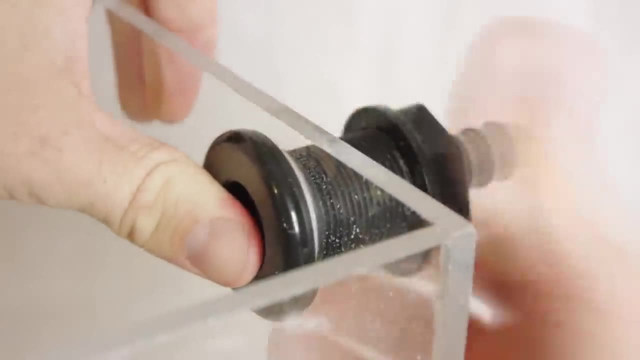 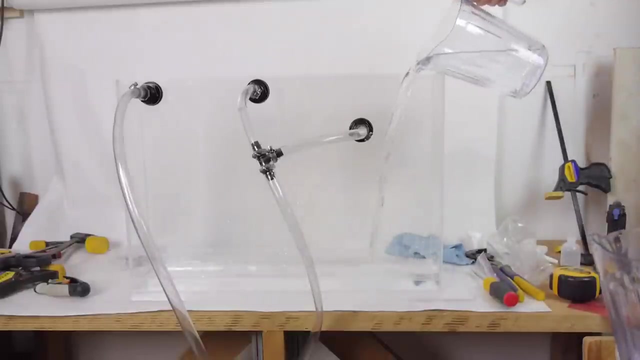 made of quarter-inch acrylic sheets cut to size on the table saw. Solvent welding is used to connect the acrylic sheets into a narrow box. All of the plumbing is composed of aquarium bulkhead fittings and clear nylon tubing. Everything was leak tested before the sand was added. Here's how it works. Potassium permanganate. 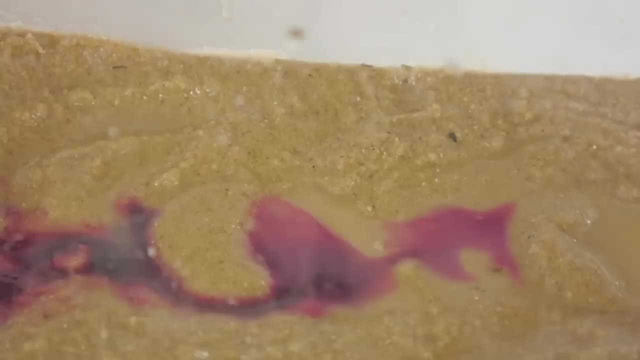 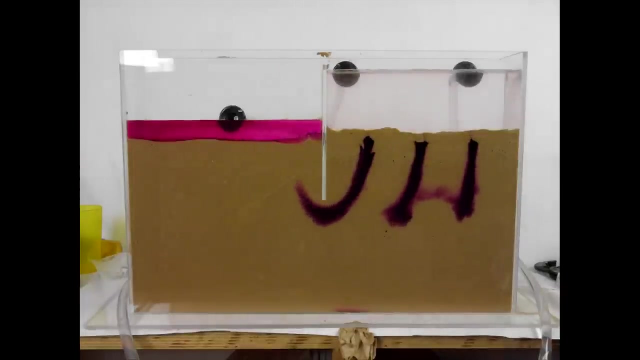 is added to three spots in the top of the sand. A pump in a bucket below keeps a constant head pressure on one side of the model. The differential between the water level in both sides is what drives the water to flow from one side to the other. Groundwater flowing through the sand creates. 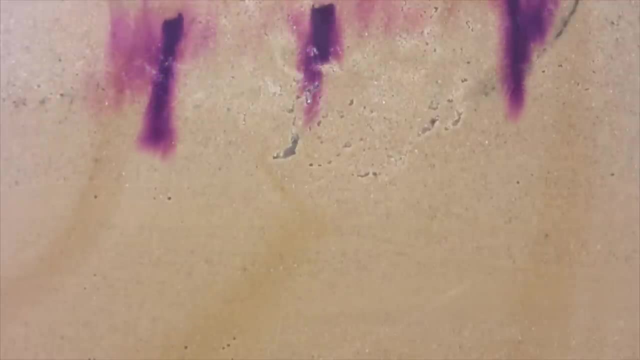 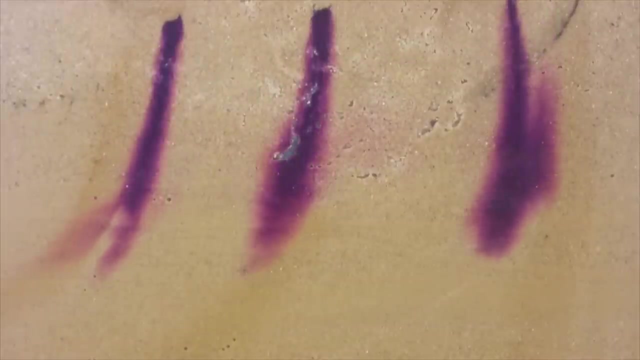 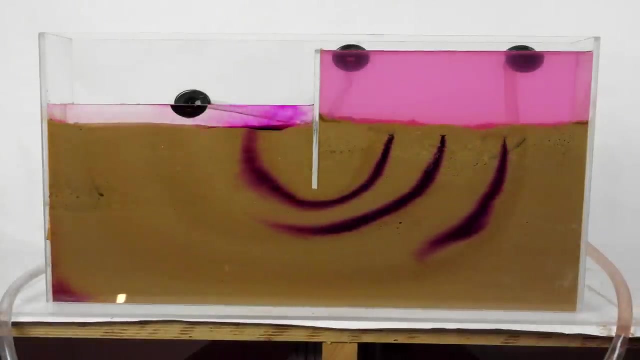 traces of the flow lines over the course of several hours, illustrating exactly what we estimated earlier. with the flow net, The flow of groundwater has an overall effect on the geotechnical process and has always been so well understood. In fact, for some states, regulation of the pumping of groundwater is established on explicit 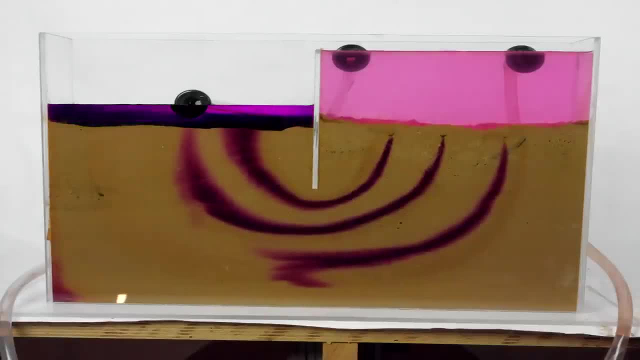 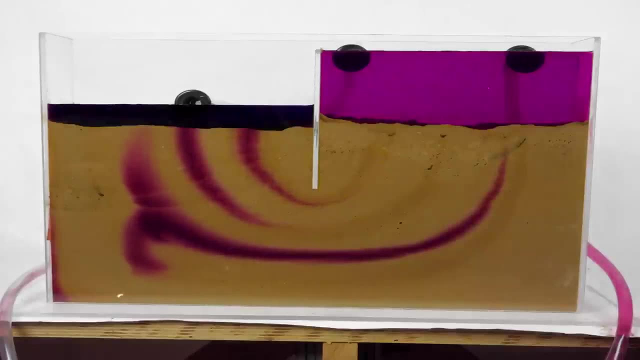 ignorance of its behavior. In a landmark case which submitted the Rule of Capture into Texas Water Law in 1904, the court said that groundwater movements are so secret, occult and concealed that regulating the use of groundwater would be practically impossible. Fortunately, geotechnical.